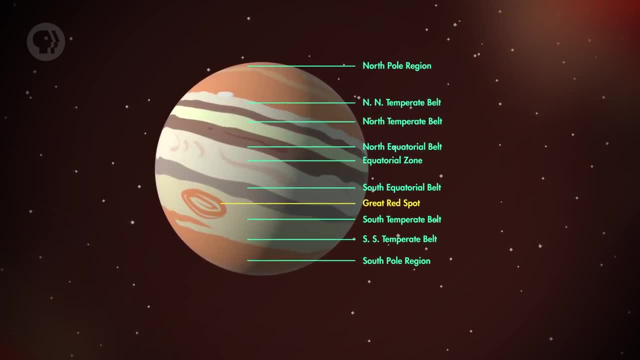 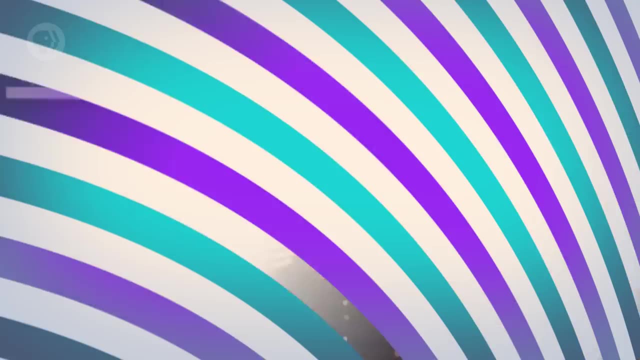 with multiple stripes running parallel to its equator. The lighter color stripes are called zones and the darker ones belts. They're fairly stable, though their shape and coloring change over time. Belts and zones circulate around the planet in opposite directions. They form due to the 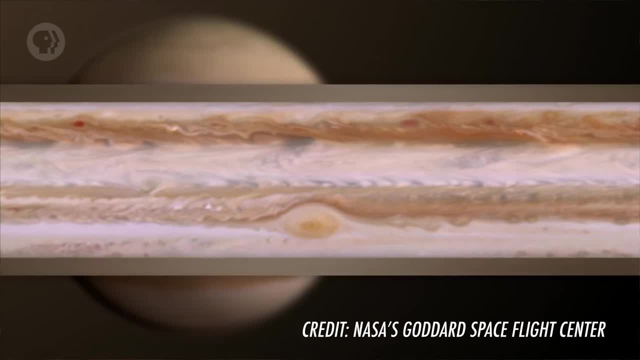 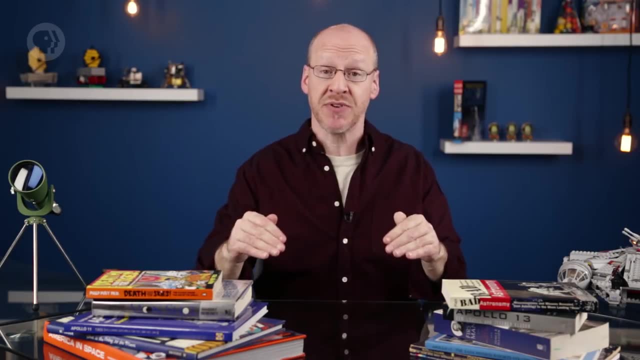 convection in Jupiter's atmosphere. Upwelling air cools and forms white ammonia clouds. That creates the light-colored zones That air flows to the sides and sinks, and sunlight changes the chemistry in the clouds, forming molecules that color the air yellow red. 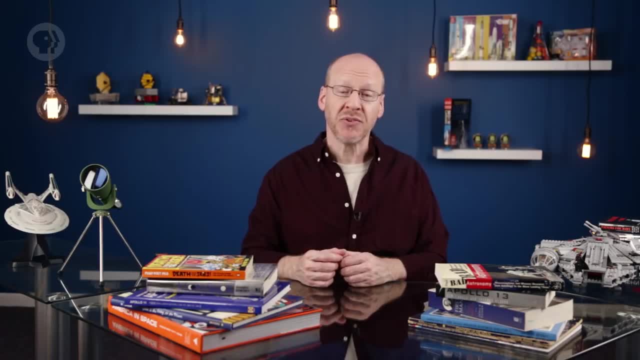 and brown. This is what causes the darker belts. In May of 2010,, one of Jupiter's biggest belts sank so deeply it disappeared from view, completely covered by other clouds. Then, a few months later, it popped back up and reappeared, none the worse for wear. This has happened several times in the past, too. 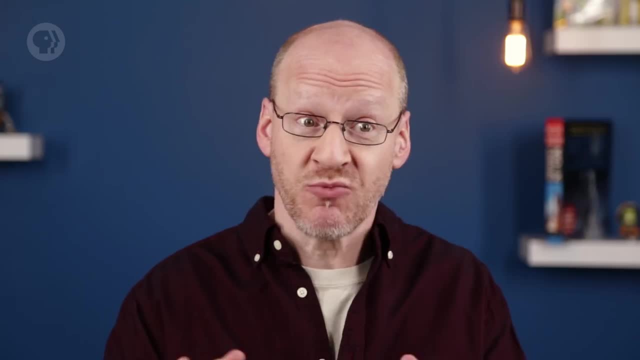 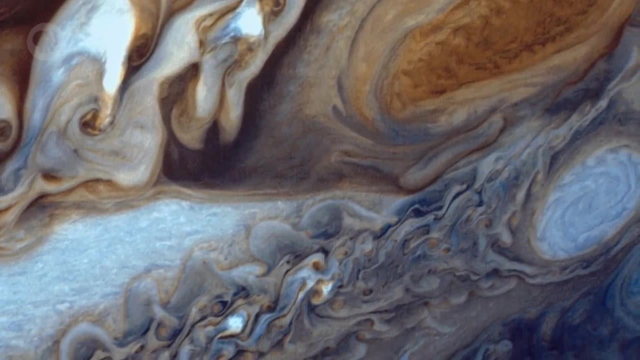 I saw one of these events once through a telescope, and Jupiter looked really weird. lopsided Turbulence in the regions between zones and belts can create storms, gigantic vortices raging in the clouds. Dozens of them dot the face of Jupiter all the time. But 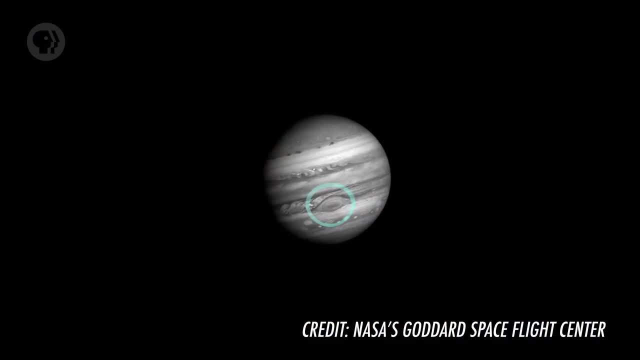 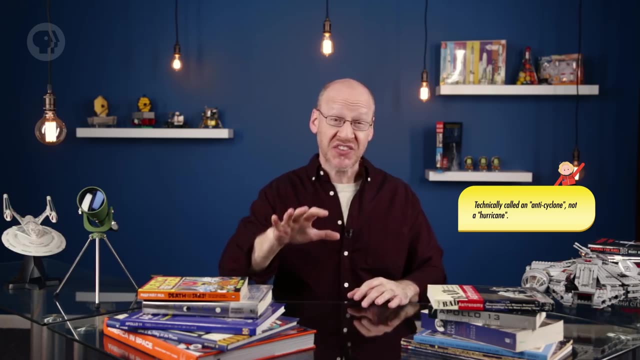 there is one to rule them all: the Great Red Spot, a fittingly huge storm for a giant planet. It's actually a colossal hurricane, several times larger than our entire planet Earth, with sustained wind speeds of 500 kilometers per hour. And it's old: It was first seen. 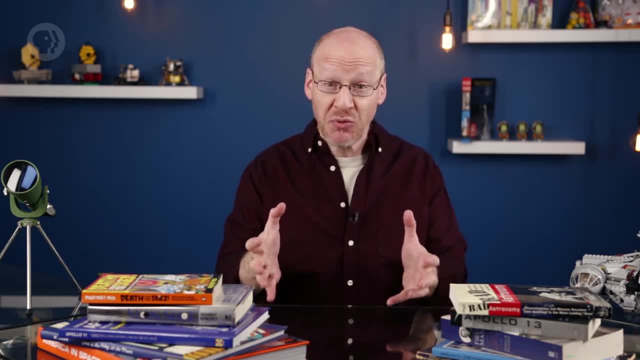 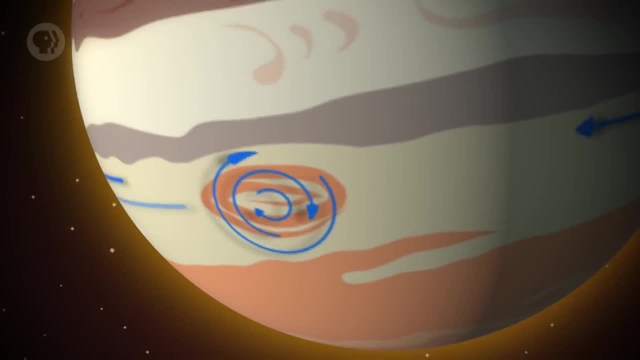 in the late 17th century. Imagine a storm on Earth lasting for more than three centuries, And it may be far older — the 1600s is just when we first spotted it. So why is it so stable? It turns out that a vortex, a local spinning region in a fluid, can persist if the fluid 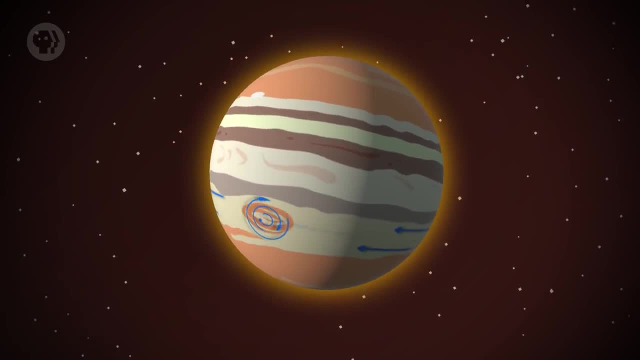 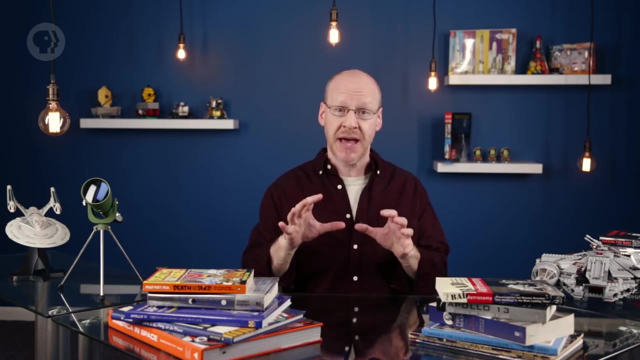 in which it's embedded is itself rotating. Jupiter's rapid spin is what keeps the red spot circulating, And the redness is probably due to cyanide-like molecules that absorb blue light, letting redder light pass through. Weirdly, the red spot appears to be shrinking. 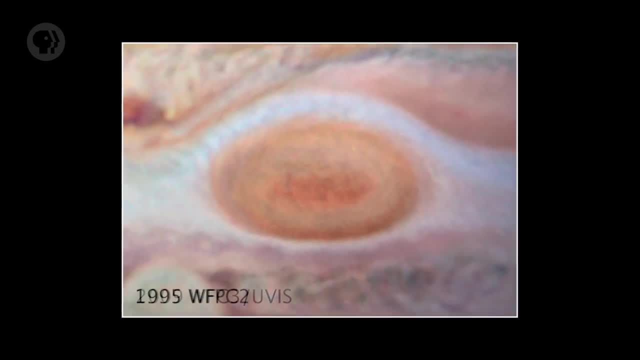 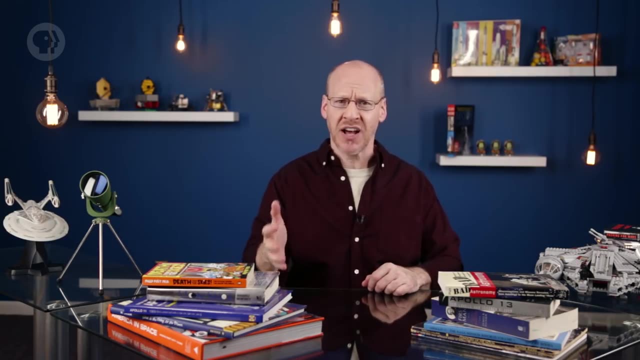 It was substantially bigger and more elongated just a few decades ago. It changes color over time too, having gone from deep red to salmon and then back again. No one knows why its shape, size and color change, But given how long the spot's been around, I doubt it's going to evaporate any time. 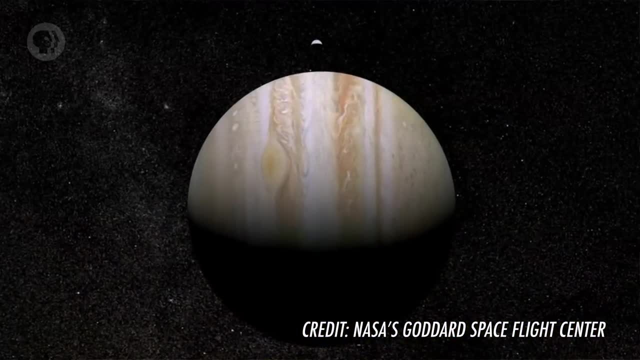 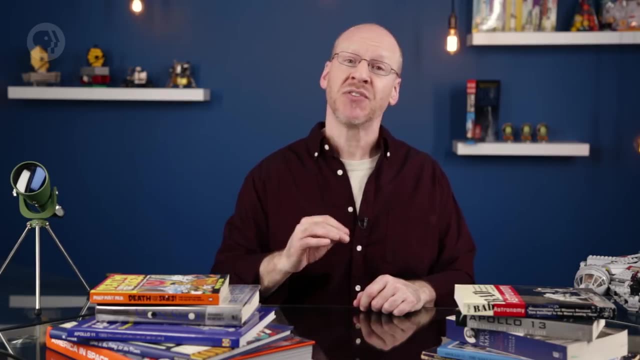 soon. Remember, we're only seeing the tops of the clouds on Jupiter. Its atmosphere is thick, several hundred kilometers deep, Like the composition of the Sun. the air on Jupiter is mostly hydrogen and helium, but it's also laced with ammonia, methane and other. 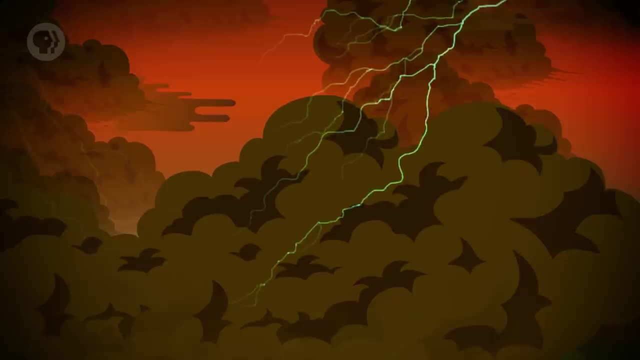 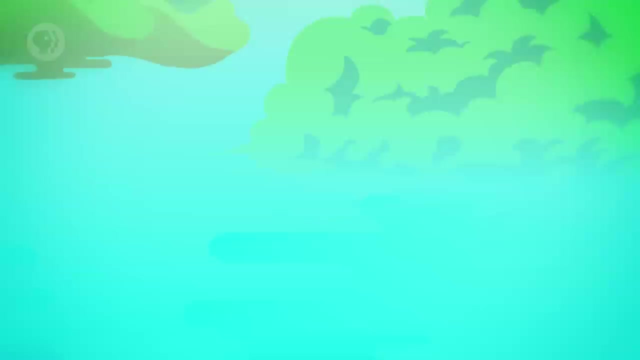 poisonous gases. As you dive into Jupiter's atmosphere, the pressure increases with depth, But you'll never reach the surface. The planet doesn't really have a proper surface. The gas gets thicker and hotter and eventually just sort of smoothly changes into a liquid. 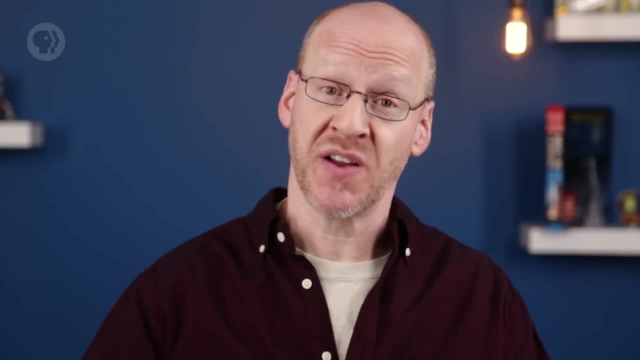 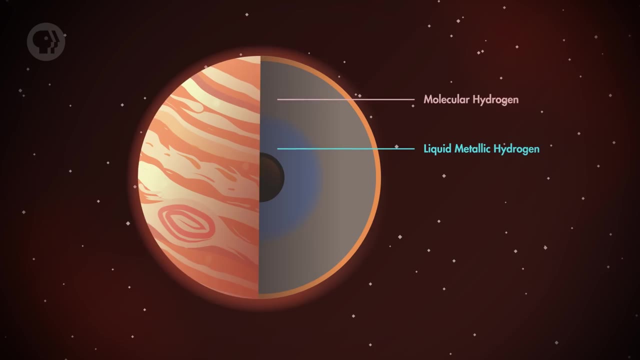 over a several hundred kilometer range below the clouds Below. that is where things get really weird. Instead of a mantle, like terrestrial planets, Jupiter has a huge region made up of liquid metallic hydrogen. We think of hydrogen as being a gas or, if it gets really, 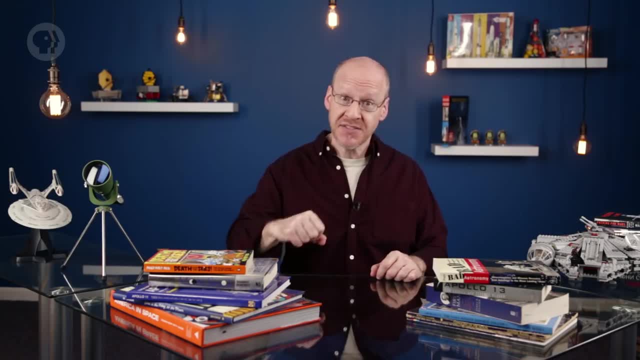 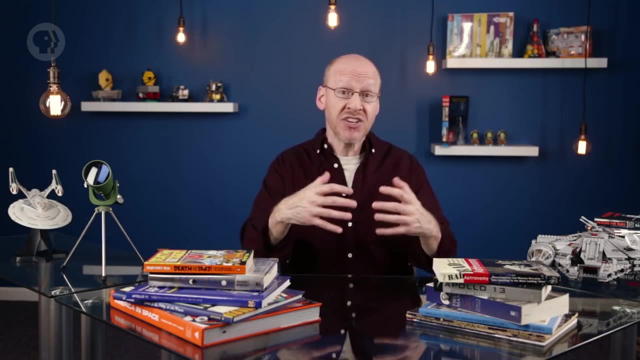 cold a liquid. But under the ridiculous pressures generated deep inside Jupiter, hydrogen undergoes this strange transformation. Individual atoms don't hold onto their electrons, but instead share them. This means the hydrogen can conduct electricity and has other properties more like a metal. 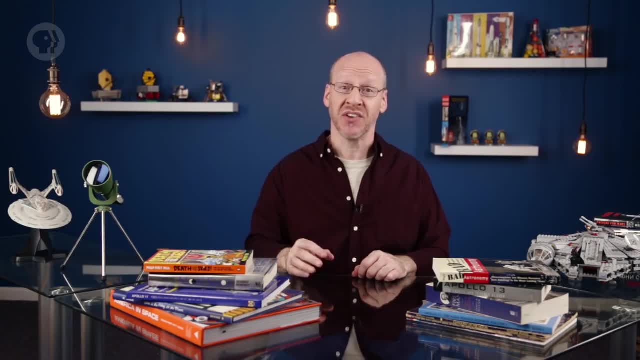 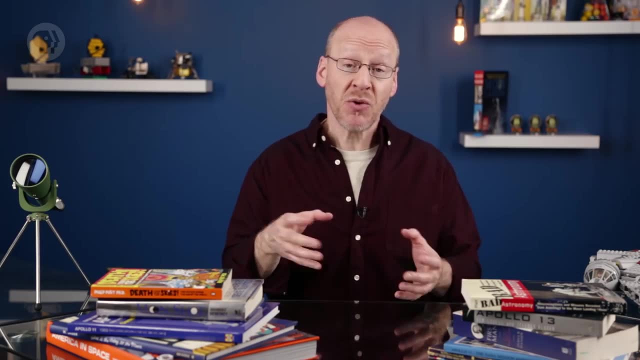 This substance is hot too, About 10,000 degrees Celsius hotter than the surface of the Sun. If we could see it, it would glow tremendously bright. Finally, at its center is most likely a dense core of material, probably composed of rock and metal. 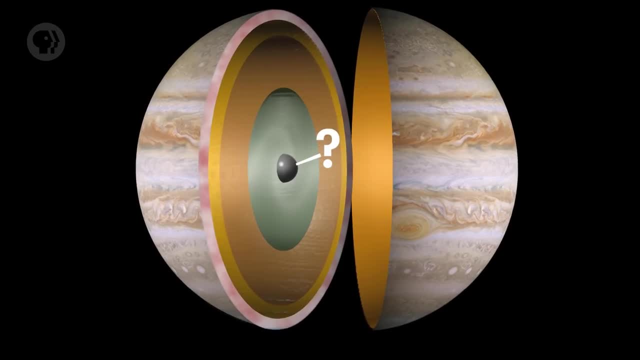 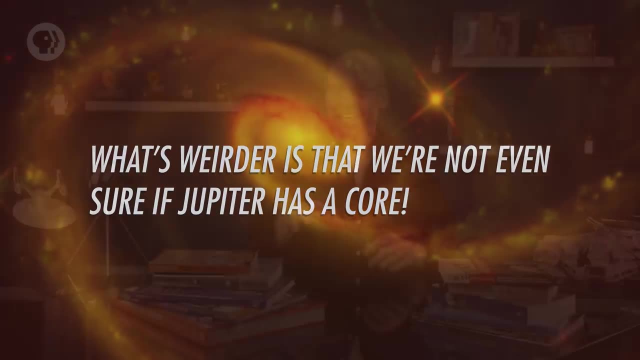 We really don't know, because it's incredibly difficult to understand the physics and chemistry locked in at those pressures and temperatures. What's weirder is that we're not even sure if Jupiter has a core. If it did, it's possible it was eroded away by currents of hot metallic hydrogen early on in Jupiter's. 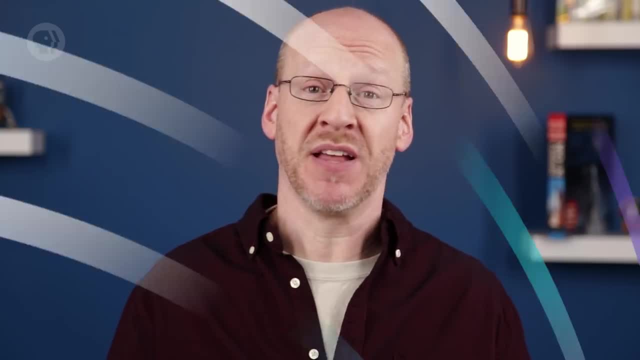 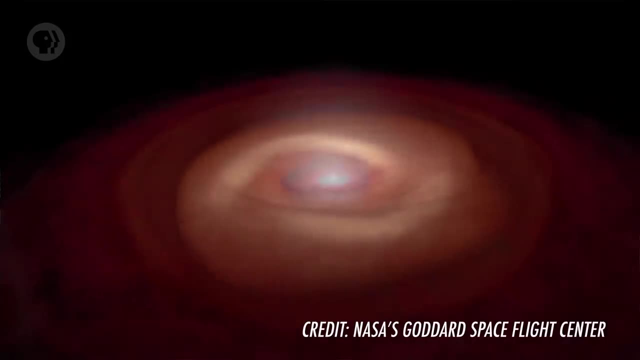 formation process. It's also possible it never had a core in the first place. The solar system formed from a flat disk of gas and dust. The center of this disk is where the Sun was born, and it's thought that the planets formed as smaller particles of 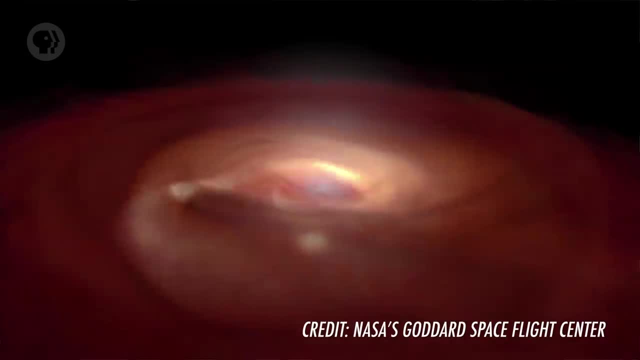 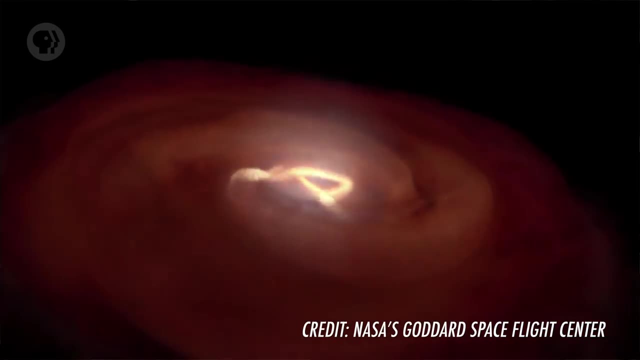 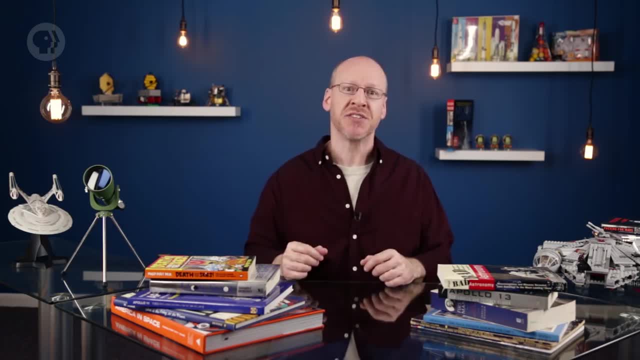 them due to their gravity. Jupiter formed where the disk was thick, rich with material. It's possible that several large protoplanets were forming, collided and stuck together to really kickstart Jupiter's growth. If that were the case, it started out with a rocky metallic core and once it, 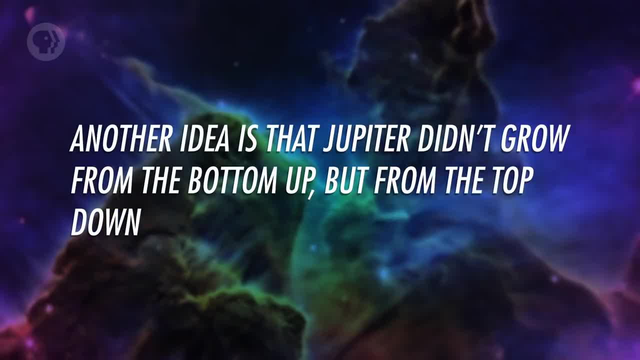 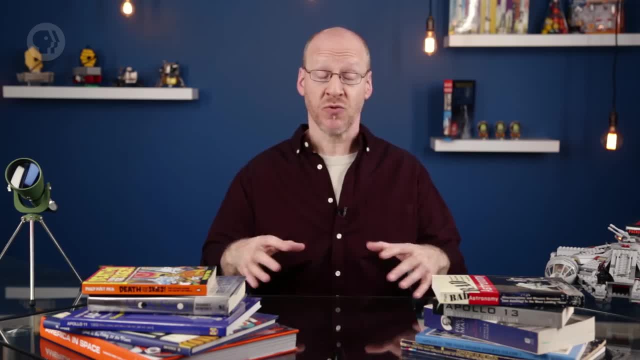 got big enough, it drew in that gas that made it the giant we see today. Another idea is that Jupiter didn't grow from the bottom up, but from the top down. The disk itself collapsed in several places to form huge distended clumps. 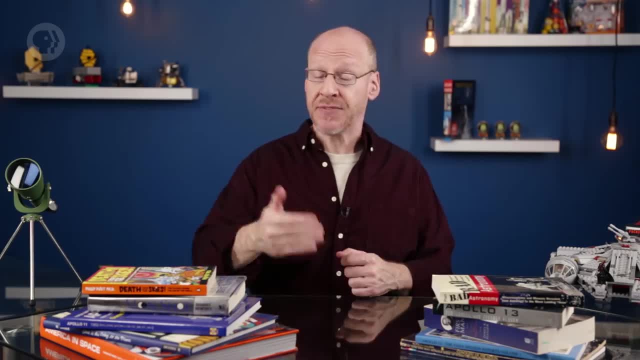 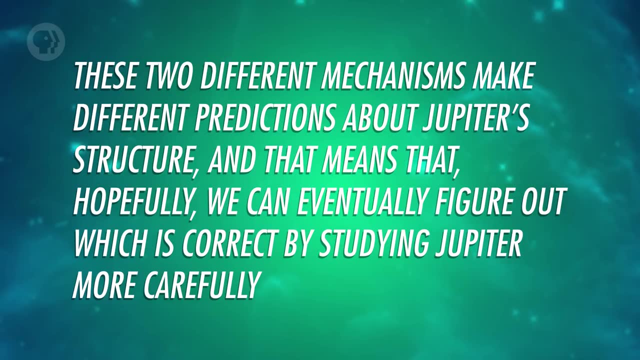 These then would have collided, stuck and created the planet. If that's the case, then Jupiter might not have a core at all. These two different mechanisms make different predictions about Jupiter's structure, and that means that hopefully, we can eventually figure out which is correct by studying Jupiter. 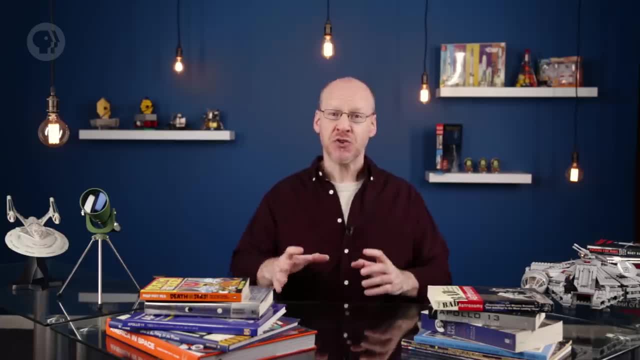 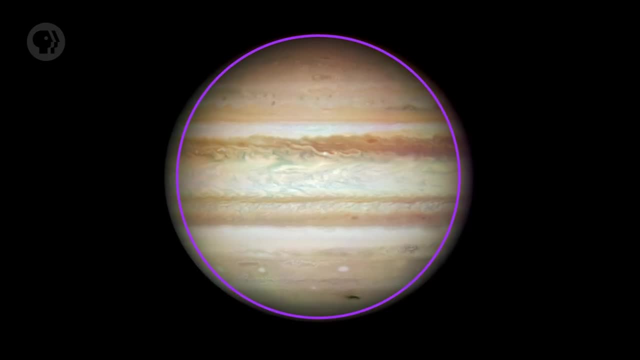 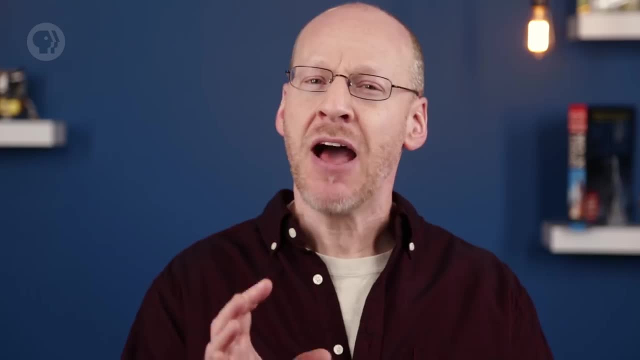 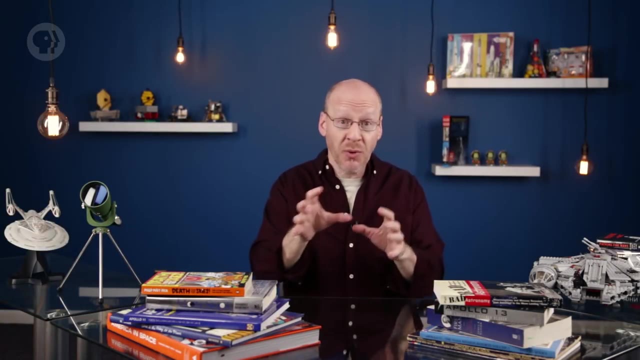 as it used to be. So Jupiter is a big bruiser of a planet, But how close was it to becoming a star? Sometimes people ask me if Jupiter is a failed star. In other words, as it formed, it almost got massive enough that nuclear fusion could start in its center, turning it into a star. 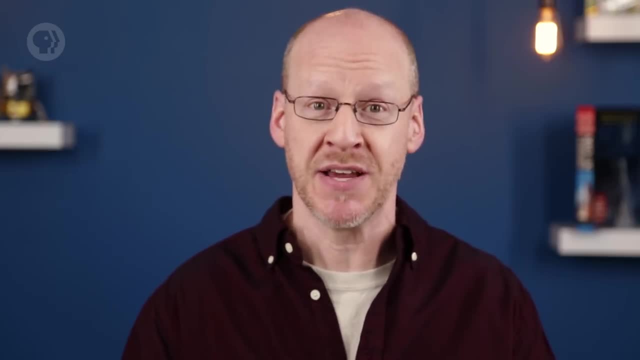 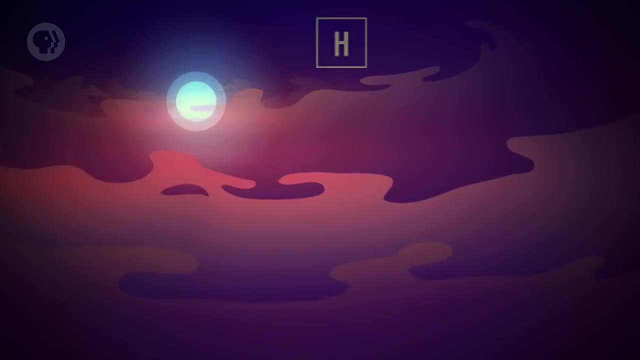 I see this a lot on TV shows and in articles and it really burns me up. When a star forms, hydrogen fusion starts when the star gathers so much mass that its gravity can compress atoms together in its core hard enough to get them to fuse This. happens when a star has roughly one-twelfth of the Sun's mass. In fact, the smallest stars we see do have about that mass. What about Jupiter? The mass of Jupiter is about one-one-thousandth the mass of the Sun, Far too little to undergo fusion in its core. If you want to turn Jupiter into a star, you'd have a lot of work ahead of you. You'd have to take Jupiter and then add about 80 more Jupiters to it. Saying Jupiter is a failed star is really unfair. It's not a failed star, It's a. 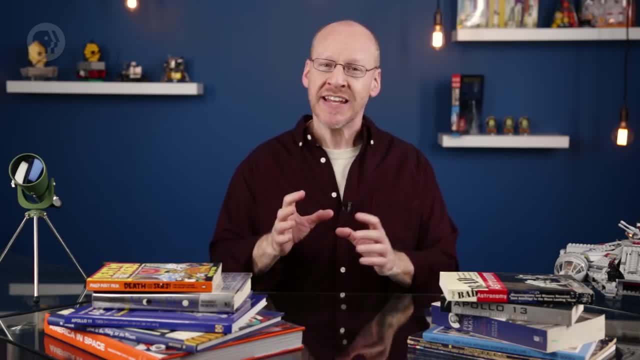 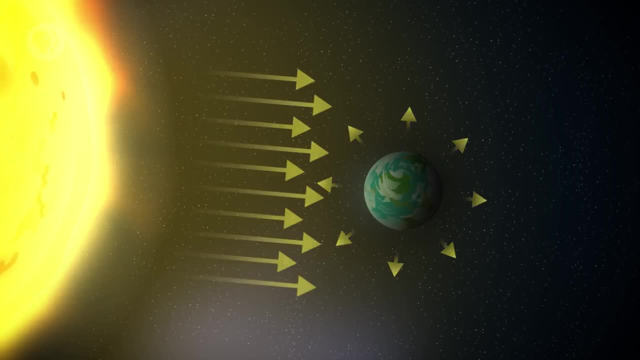 really successful planet. Even though Jupiter isn't a star, it does have another fundamental function: It's a sunny property. It emits more heat than it receives from the Sun. The Earth and other terrestrial rocky planets are in a heat balance with the Sun. We emit pretty much the same. 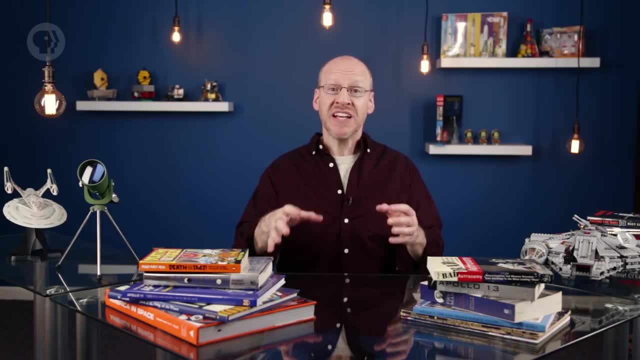 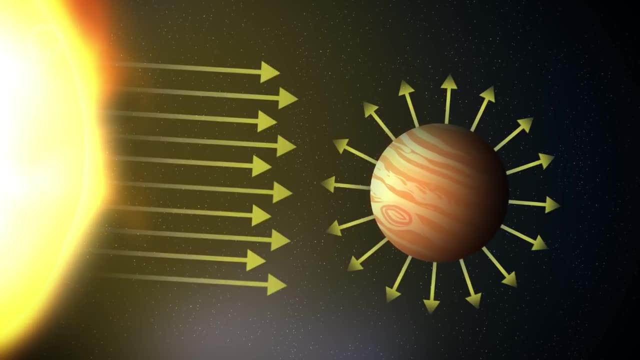 amount of heat that we receive, But Jupiter's different. After it formed, it started to cool by radiating away heat from its upper atmosphere. A large fraction of the planet is a gas, remember, and when you cool a gas it contracts. So the atmosphere cools and contracts, but this increases the. pressure inside the planet, so it heats up. That heat works its way out of Jupiter and gets radiated away as infrared light. In the end, the amount of heat Jupiter gives off is more than it receives from the Sun. It's still actively cooling 4.5 billion years after it formed. Oh and hey remember. 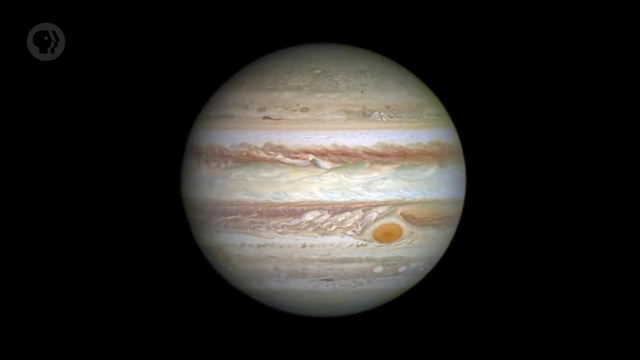 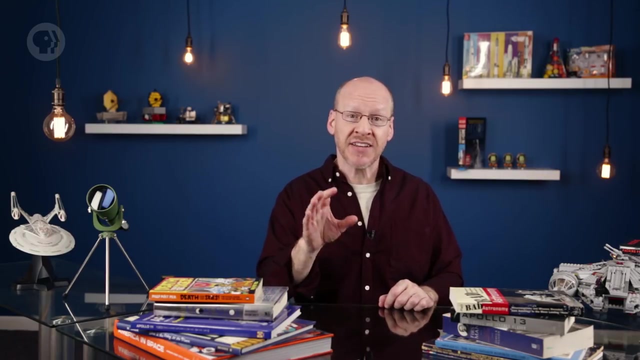 the belts and zones, the stripes we see in Jupiter's atmosphere and all the storms that pop up. Those are driven in large part by Jupiter's internal heat. On Earth our weather is powered by heat from the Sun, but on Jupiter they get their energy from the. 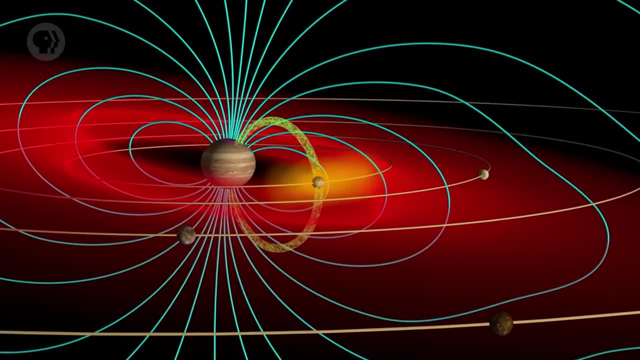 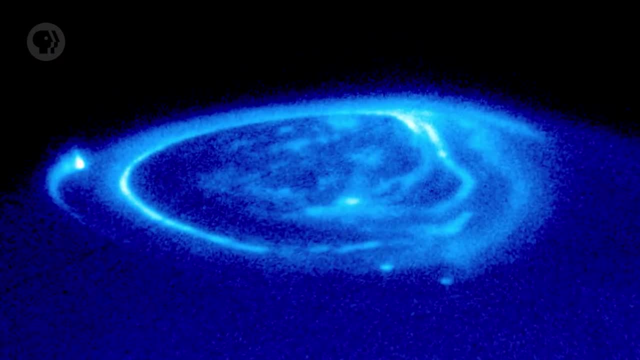 planet itself. Jupiter has a very strong magnetic field, no doubt due to all of that metallic hydrogen inside it, Coupled with its rapid rotation. Like Earth, it has aurorae at its poles as the solar wind is funneled down to the cloud tops, As we'll see next week, Jupiter's moons affect the magnetic field and aurorae on Jupiter as well. Jupiter also has a ring, though it's not nearly as grand as Saturn's. It wasn't even discovered until we sent space probes to the planet. The ring is made of dust, probably. thrown into orbit around the planet due to meteorite impacts on its smaller moons. Speaking of impacts, we know that Earth gets hit by interplanetary debris all the time. Go outside for an hour and you're bound to see a few meteors. It's larger and with more gravity, gets hit a lot more, A lot more, A lot, And sometimes it gets hellaciously whacked. In 1994, the comet Shoemaker-Levy 9 impacted Jupiter Multiple times Jupiter's fierce. 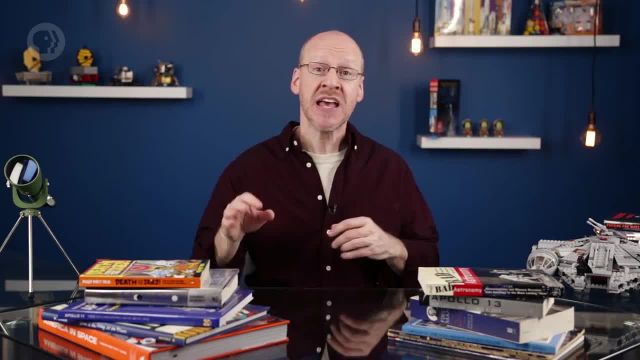 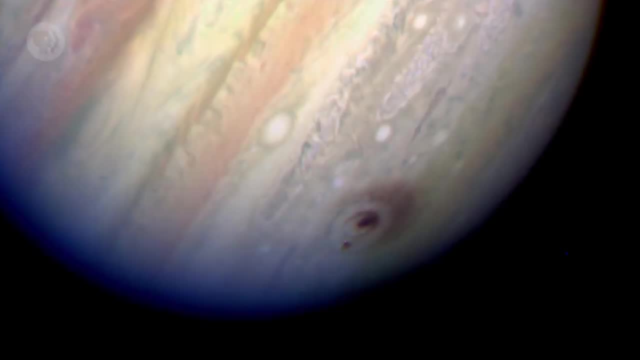 gravitational tides had ripped the comet into dozens of pieces and each slammed into the planet one after the other with the force of millions of nuclear weapons. The scars left in the upper atmosphere from the plumes of material that exploded outward lasted for. months. The comet has been in Jupiter's atmosphere since then, and it may suffer an impact large enough to see from Earth every year or so. And while that sounds scary, it might actually be our savior. There's an idea that Jupiter's gravity tends to take comets that fall toward the 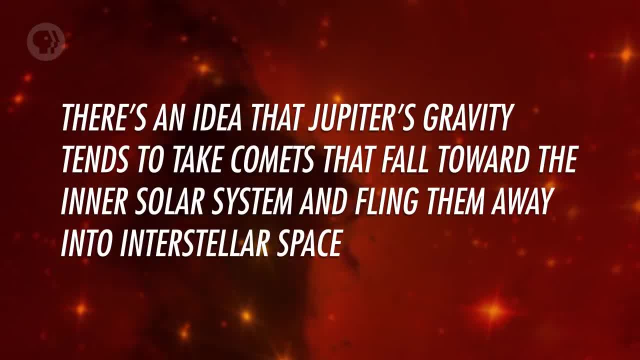 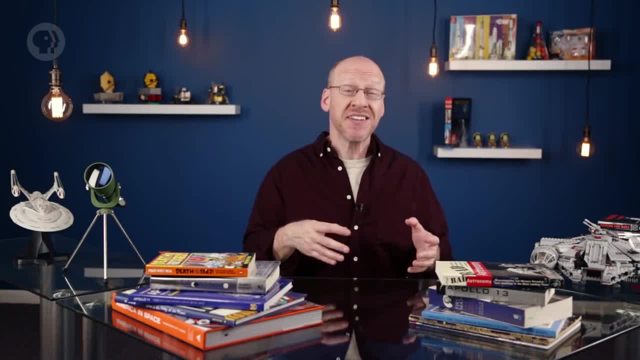 inner solar system and fling them away into interstellar space Over the eons. this has cleaned out a lot of otherwise dangerous objects that could have eventually hit Earth. On the other hand, Jupiter has a tendency to warp the orbits of some other comets, so 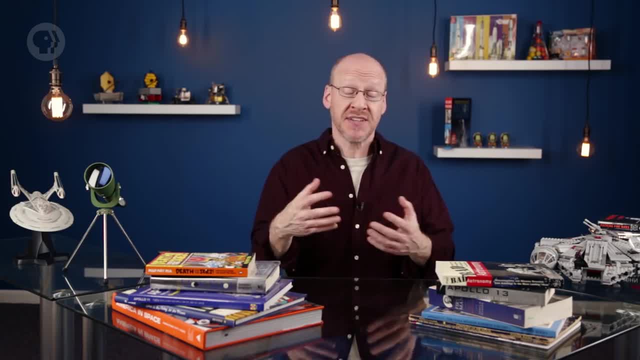 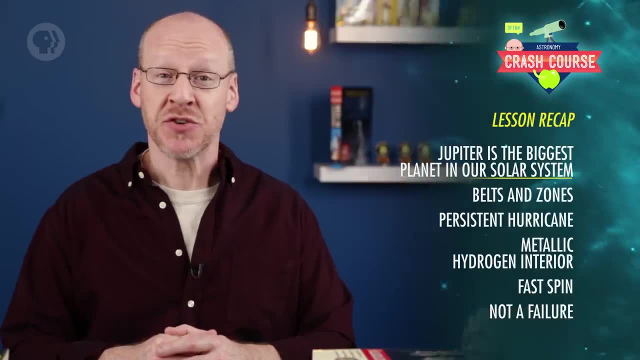 that they do swing by the Earth. Is this a net benefit or not, But either way, it's clearly the two-septillion-ton gorilla in the solar system. Today you learned that Jupiter is really, really big. It's the biggest planet in our 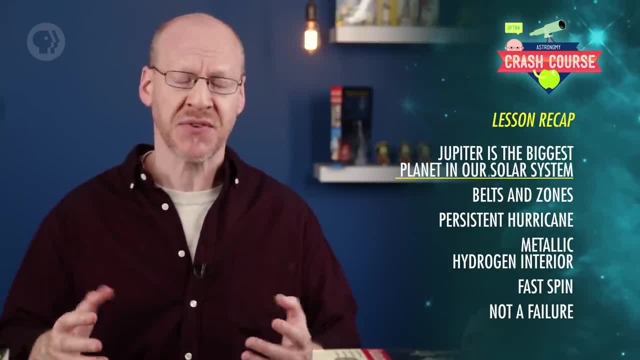 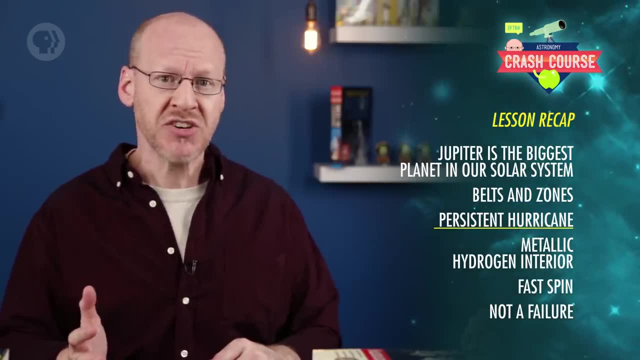 solar system, a gas giant. It has a dynamic atmosphere, including belts and zones, and a gigantic red spot that's actually a persistent hurricane. Jupiter is still warm from its formation and has an interior that's mostly metallic hydrogen, And it may not even have. 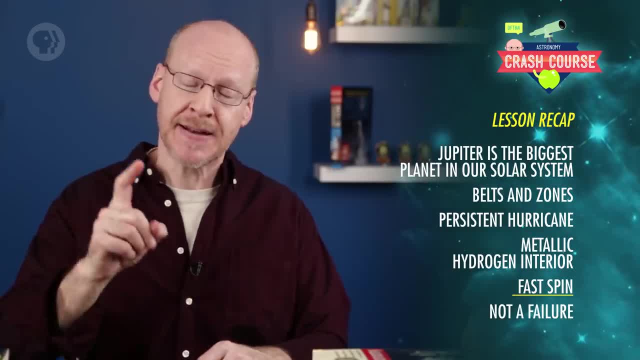 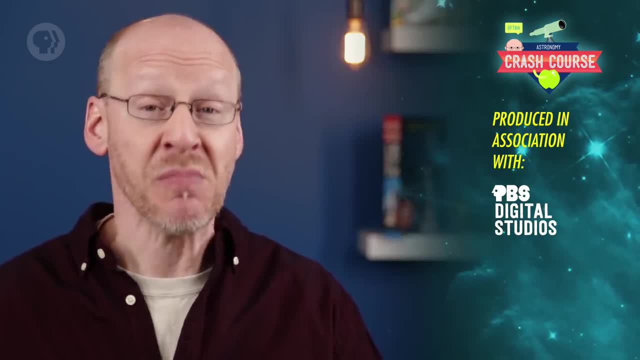 a core. It has the fastest spin of any planet and it's not a failed star. Crash course in space. Crash Course Astronomy is produced in association with PBS Digital Studios. Head on over to their channel to discover more awesome videos. This episode was written by me, Phil Plait. The script was edited by Blake DePastino. 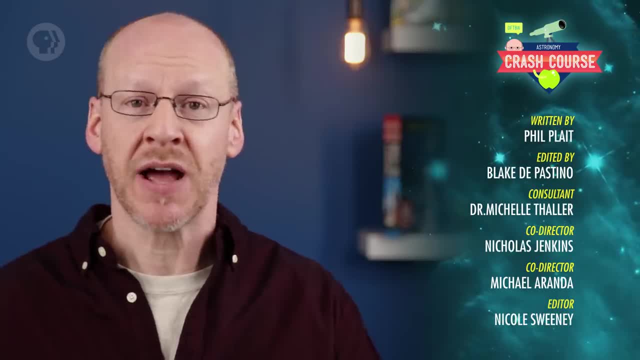 and our consultant is Dr Michelle Thaller. It was co-directed by Nicholas Jenkins and Michael Aranda, edited by Nicole Sweeney, and the graphics team is Thought Cafe.